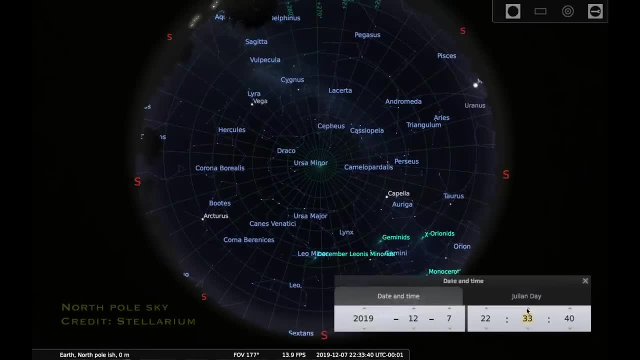 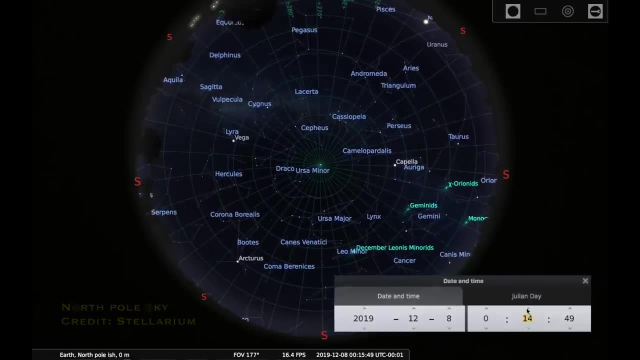 really can't appreciate it at all. And even further north up, like on the pole itself, it never rises there and you can't see it at all. So the Milky Way is kind of like a fried egg shape. right, It's a flat disc with a big bulge. 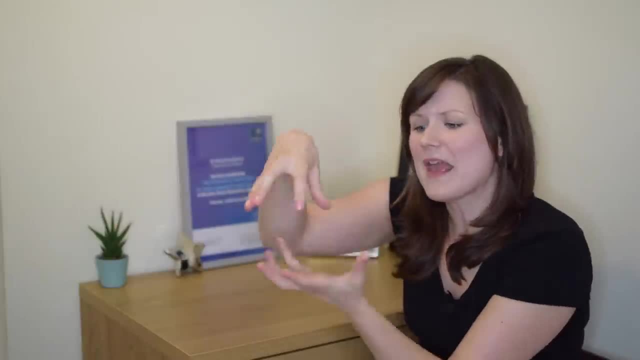 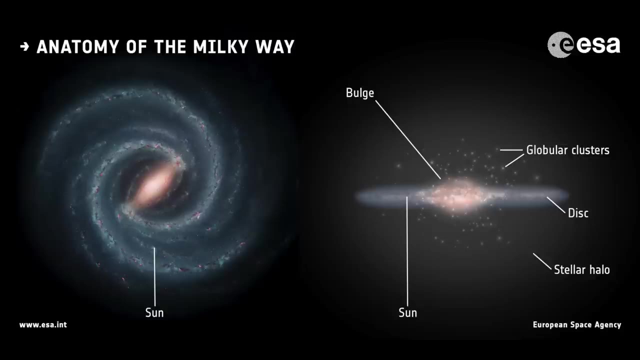 yoke in the middle where there's lots and lots of stars. there's a supermassive black hole at the centre, And if the sun is just one star in the Milky Way that orbits around the edge and we, the Earth, go around the sun, then how come is it that from the Southern Hemisphere they're the only ones? 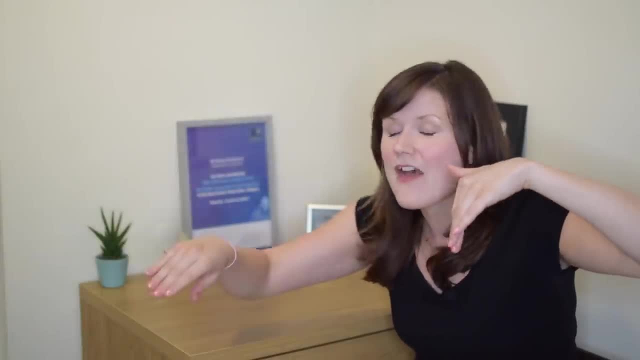 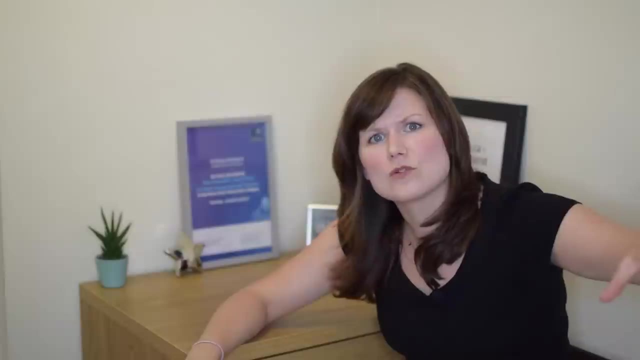 able to see the centre of the Milky Way? And if that's the case, then why is it that we, the Earth, we the centre of the Milky Way, where there's lots going on, and in the Northern Hemisphere we look out towards the edge of the Milky Way? You know, when you picture the Earth going around the sun, 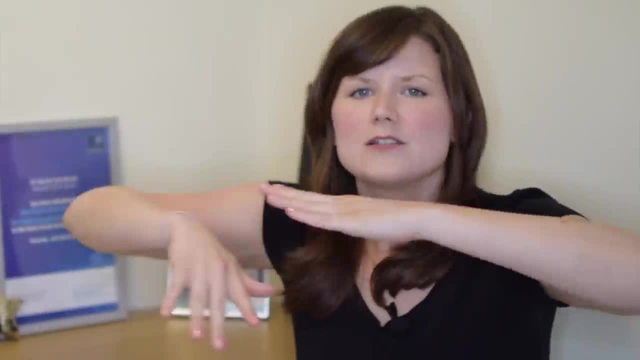 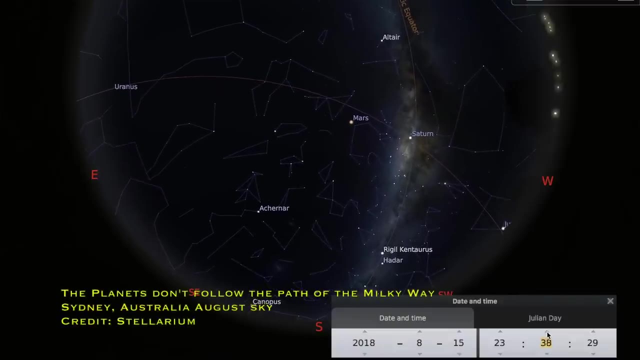 and the sun going around the Milky Way. you picture them sort of all going around in a line, But that's not true. you know, if it were, then the path of the planets, the sun, the moon, everything that's in the plane of our solar system, in the sky, would trace the same path. 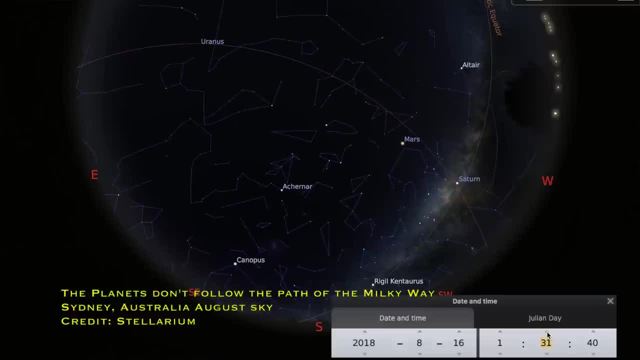 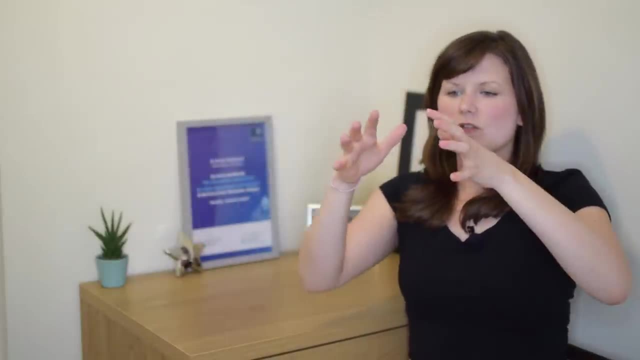 as the Milky Way does across the sky. But that's not the case. If we think about, like, how we navigate around this dive, we picture the Earth and the sky is sort of an extension of the surface of the Earth. it's in a sphere that surrounds us. Obviously it's in three dimensions. 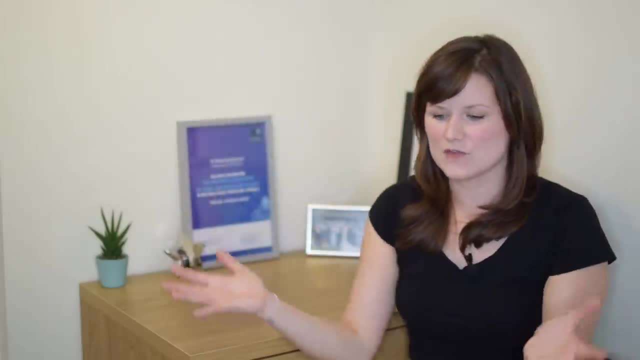 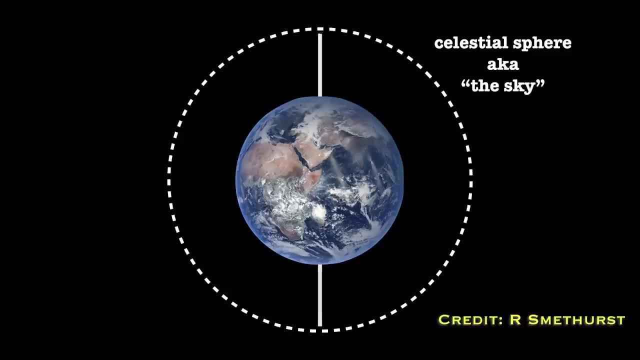 but really how our eyes perceive it, as if it's on the edge of the celestial sphere. You've obviously got the North Pole of the Earth and the South Pole of the Earth as well, And so we can imagine there's a North Pole of the celestial sphere and there's a South Pole of the celestial sphere, And 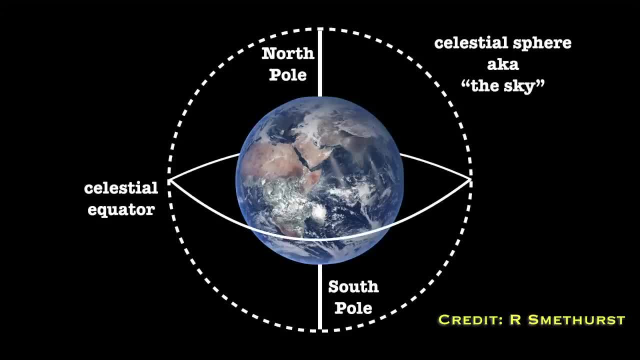 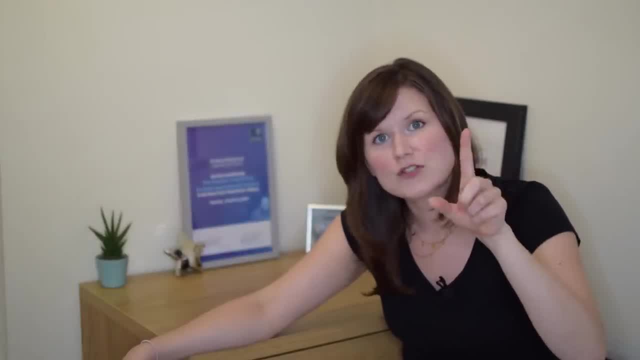 similarly, the equator of the Earth can be expanded outwards to give you the celestial equator, And it happens that the North Celestial Pole points directly at the star Polaris, the North Star, whereas the South Celestial Pole isn't actually near to any star that the human eye can actually 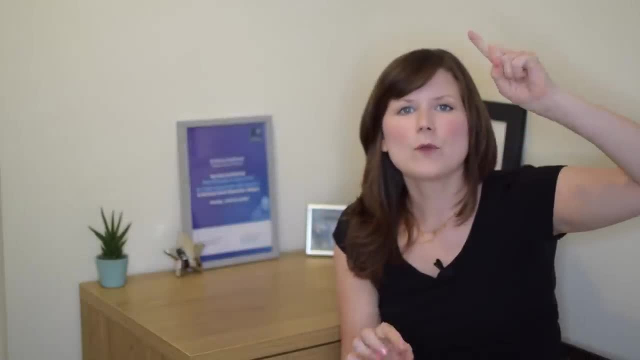 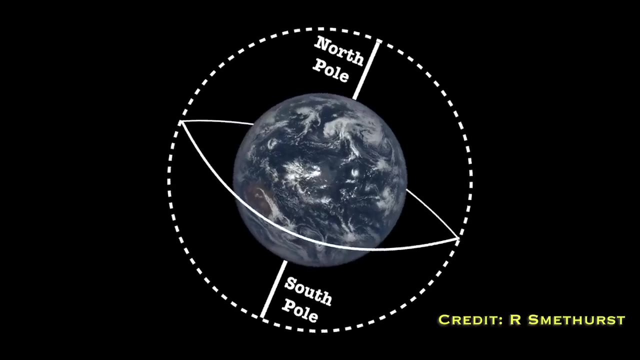 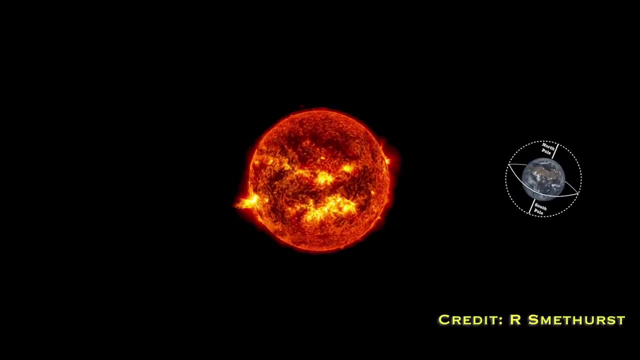 see, And the Earth spins on its axis that joins the North Pole and the South Pole. Now, the thing is that we know that that axis is tilted with respect to how we orbit around the sun. It's what causes our seasons In the Southern Hemisphere: summer, the South Pole is pointing towards the sun. 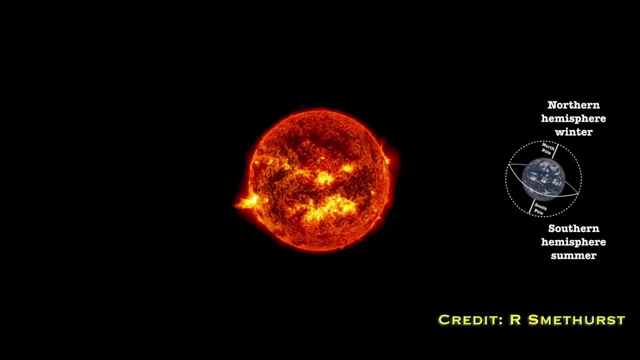 and the North Pole is pointing away, making it a little bit more difficult for us to see, And so we can imagine that the North Pole is pointing towards the sun and the South Pole is pointing away from the sun, and it's Northern Hemisphere summer and Southern Hemisphere winter Between. 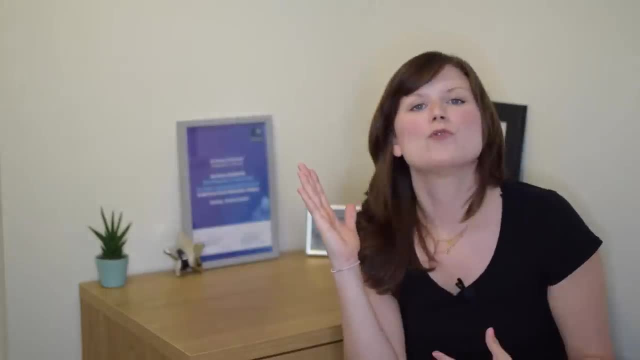 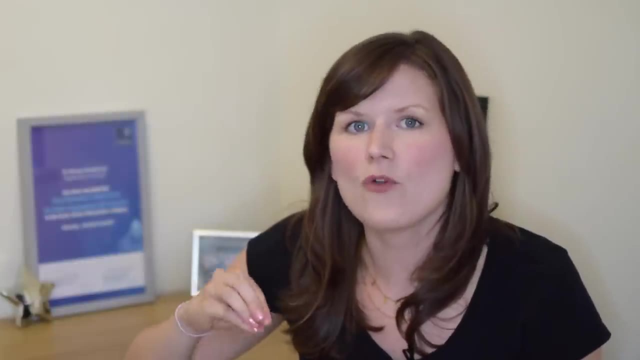 the two. you have the equinoxes- equal day and equal night- for both Northern and Southern Hemispheres, And so you have sort of autumn and spring switched around between the two hemispheres. What that means is that you've got another way of navigating around the sky Instead. 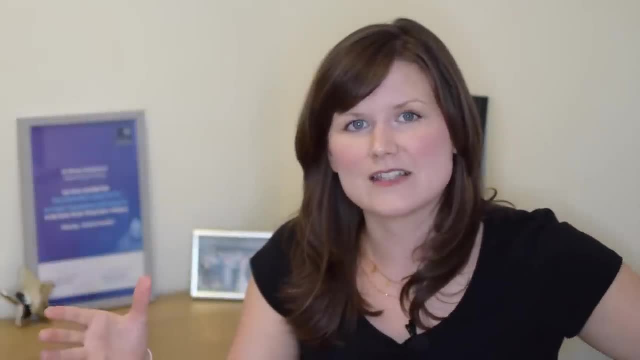 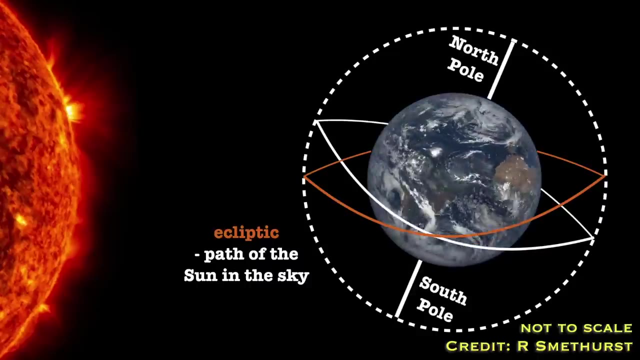 of taking the equator of the Earth and expanding that outwards to your celestial sphere. you can orbit the Earth around the sun and expand that outwards, And then you'll have a new circle around your celestial sphere, which we call the ecliptic, which is at the same angle as the Earth's. 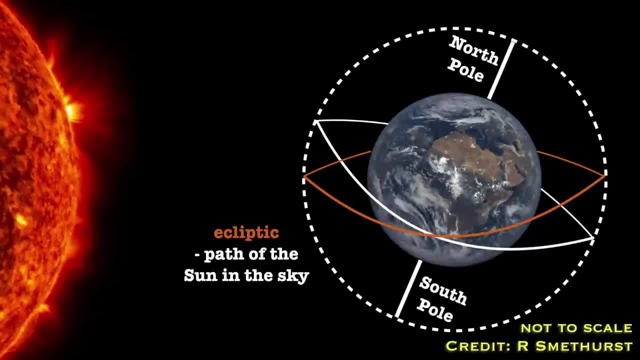 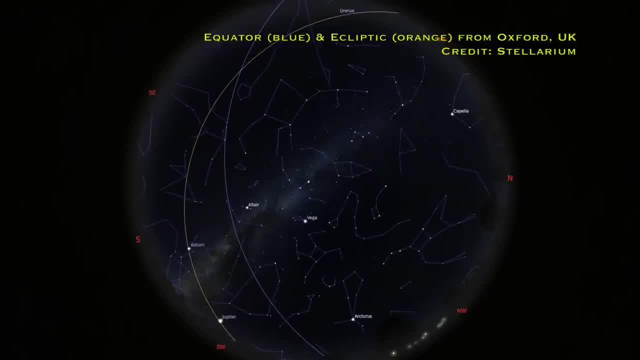 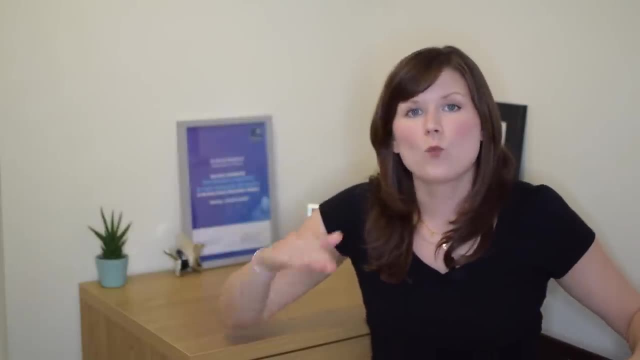 tilt of its axis with respect to the celestial equator, And that is the path that the sun and all the planets in the solar system take through the sky, because they all orbit on that same plane, around the sun. And so, along with the Earth's orbit around the sun in one plane, you've also got 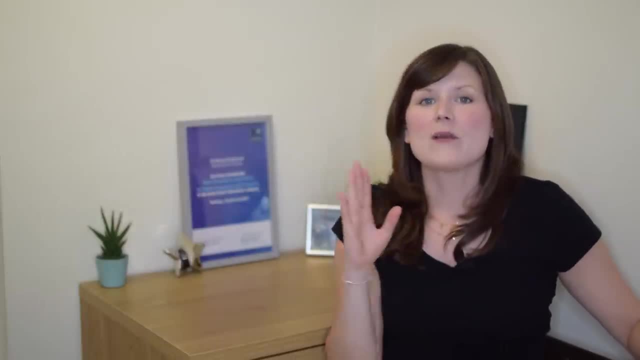 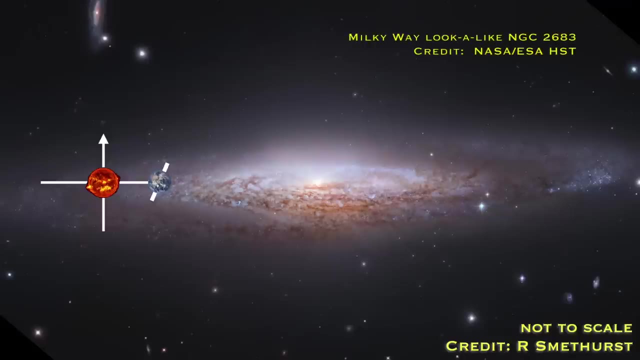 the sun's orbit around the galaxy. Now it's going around what we call the galactic plane, that plane of the Milky Way disc. But just like how the Earth's axis is tilted with respect to the plane, it goes around the sun, the sun's axis is tilted with respect to how it goes around the galaxy. And 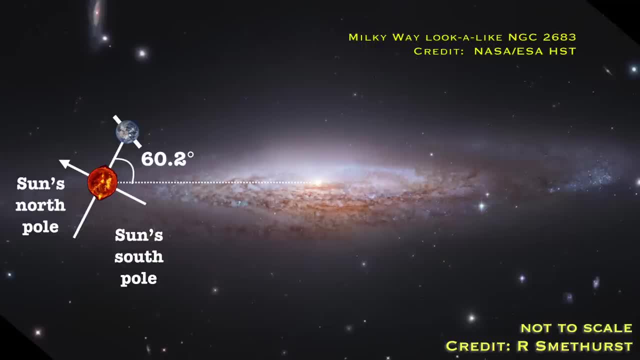 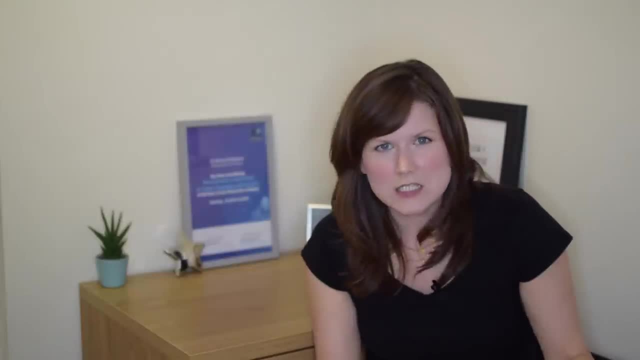 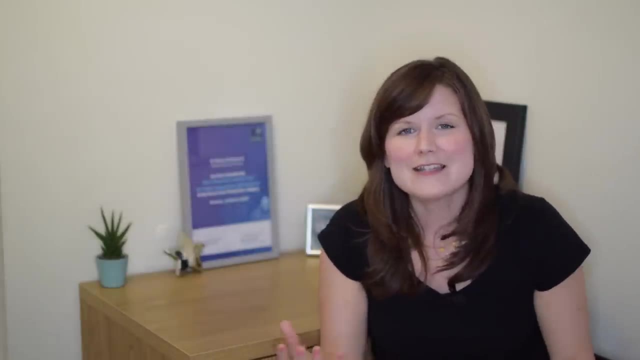 it means that the entire plane of the solar system is at an angle of about 60 degrees with respect to the galaxy. Now you might think that's really weird, that the plane of the solar system doesn't line up with the plane of the galaxy, but the two were formed independently. The galaxy is much. older than the solar system itself, and so it all just depends on what random direction the gas that made them was swirling out. So the gas that made your galaxy form and the gas that your sun and your planets formed from happened to have some rotational energy that we call angular momentum. that happened. 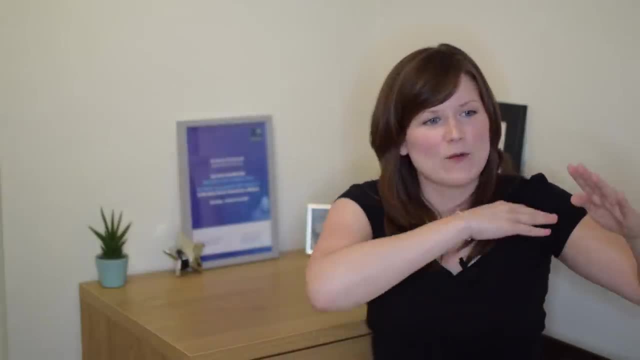 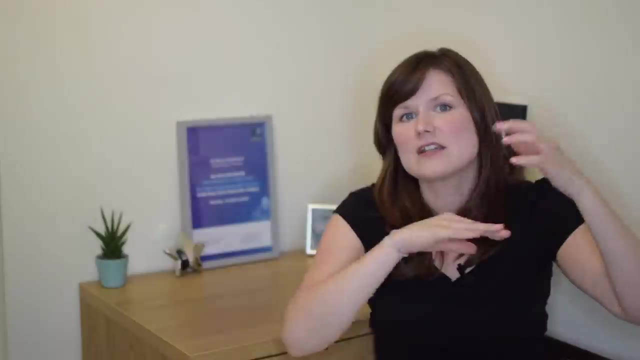 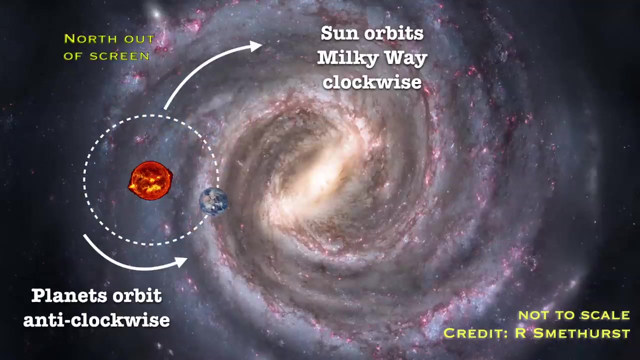 in some direction, And so that's why it ends up forming around, whatever direction that gas was going in. So for the sun, it was tilted at slightly, about 60 degrees from the rest of the galaxy And, interestingly, although those planets are going around the sun in one direction all together, 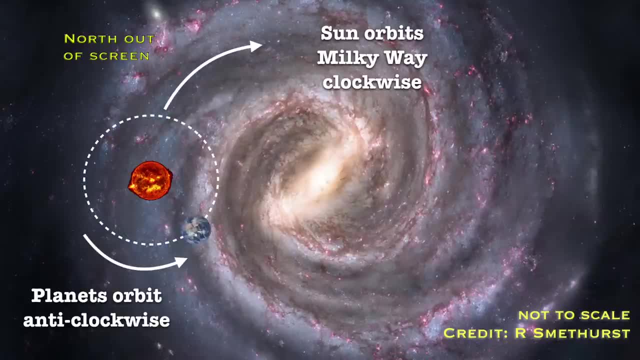 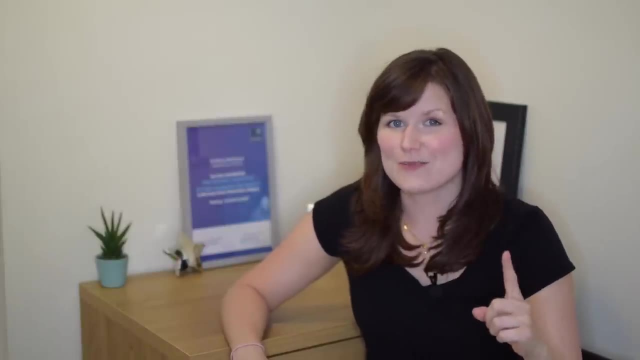 because they all form from that same cloud of gas that had the angular momentum. the sun orbits the Milky Way in the opposite direction that the Earth orbits the sun, And again it's all down to the momentum of the thing that it was formed from. So because the plane of the solar system is tilted, 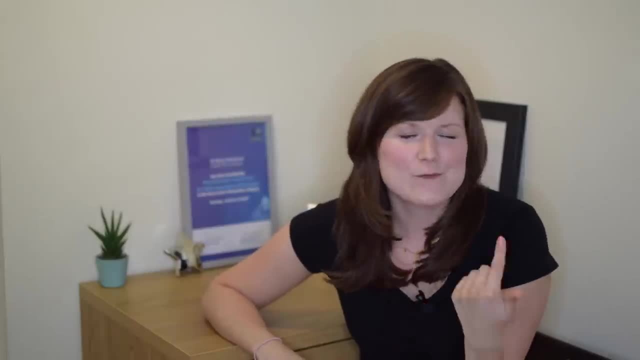 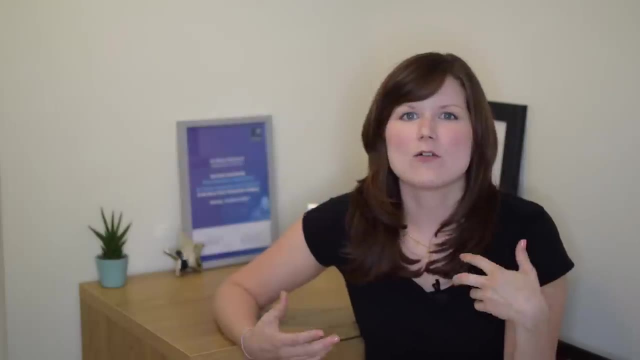 with respect to the galaxy. all hope is not lost for me, the northern hemisphere astronomer, Because, just like how the Earth's axis is tilted and it means that it causes our seasons, so that once a year the southern hemisphere points towards the sun and once a year the northern hemisphere points, 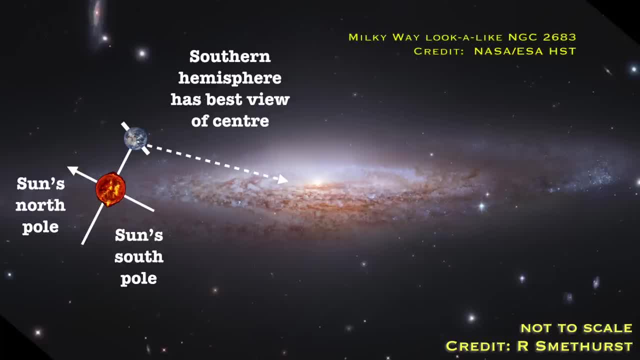 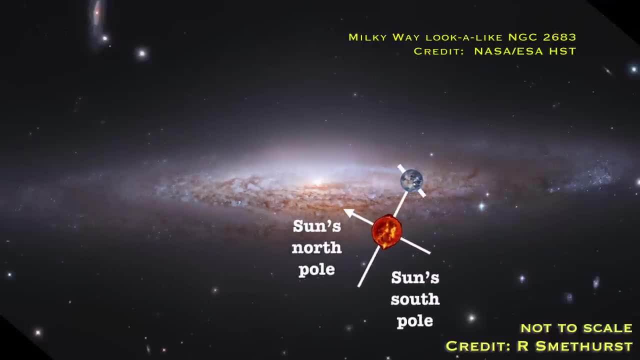 towards the sun. So as the sun orbits around the Milky Way, currently the south pole of the sun points towards the galactic centre, But as it moves around, as it's on the opposite side, it means the north pole of the sun will point towards the galactic centre. 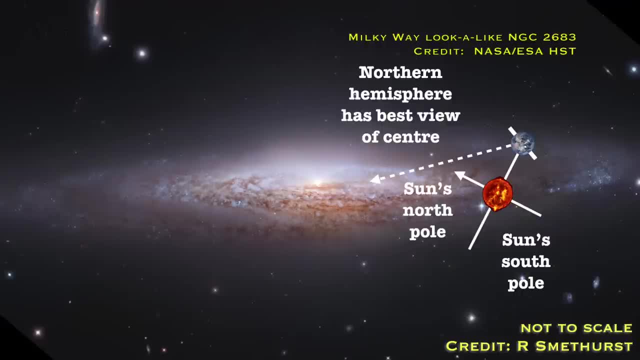 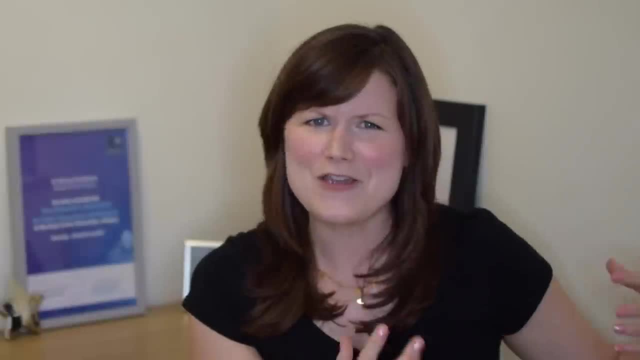 And because the tilt of the Earth means the north pole of the Earth is only about 23 degrees out from that, the northern hemisphere will point towards the galactic centre. So I guess how you can think of it is that we're currently in the sun's southern hemisphere, galactic summer and then eventually, we'll be in the sun's northern hemisphere galactic summer. The key word, though, there is eventually, because it takes the sun 200 to 250 million years to make one lap around the Milky Way, ie, its galactic year is about 250 million earth years, So we're gonna have to wait at least. 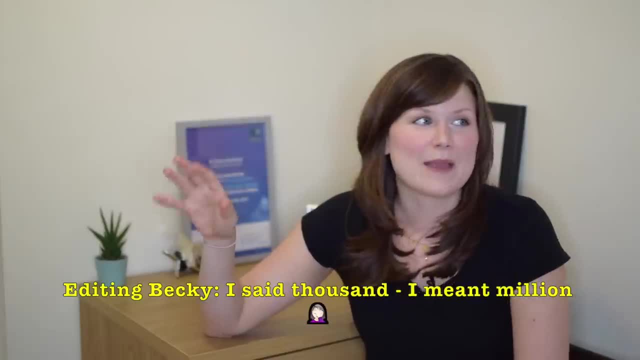 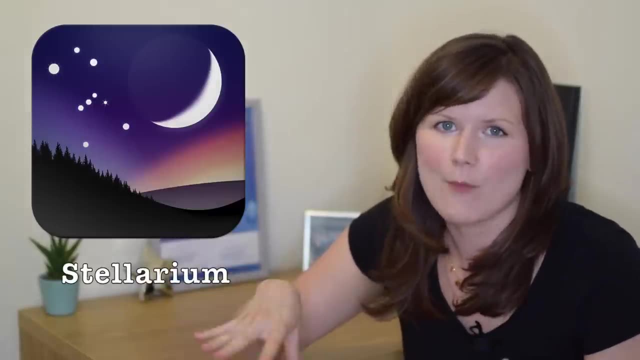 100 to 125,000 years to make it into the sun's northern hemisphere galactic summer. So I went onto Stellarium, which is this amazing app that you can get for your computer to see. you know what the sky looks like at any. 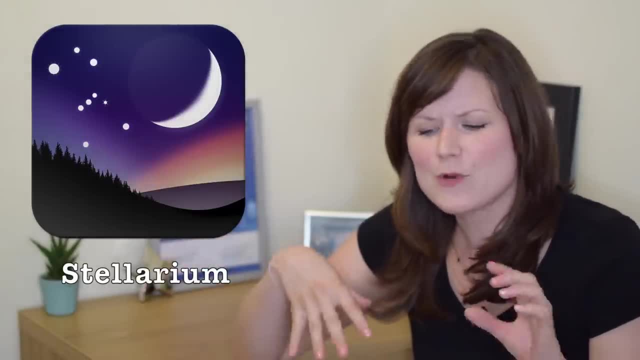 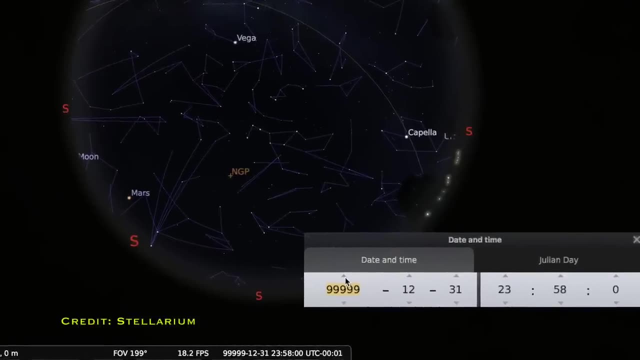 of the year, at any time of day, from anywhere in the world, and i wondered: how far in the future could it actually show me? unfortunately, stellarium only goes up to a hundred thousand years in the future, no matter how many times i clicked it to try and make it go above that a hundred thousand. 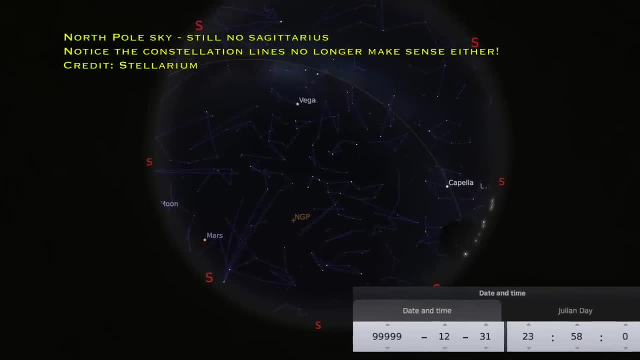 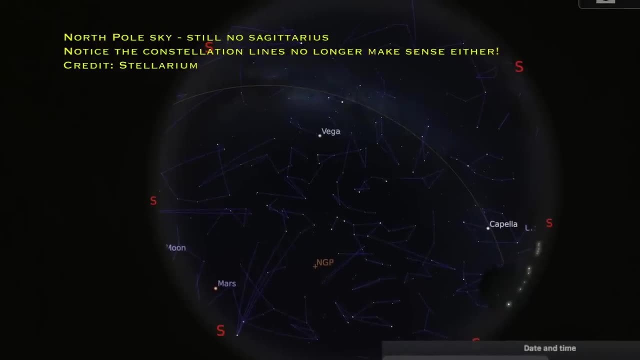 years in the future, though, sagittarius is still not visible from the north pole, and that's because the sun is only like 0.04 percent of the way around its galactic orbit. that takes 250 million years or so. it'll only be when the sun is 25 around its galactic orbit that sagittarius will 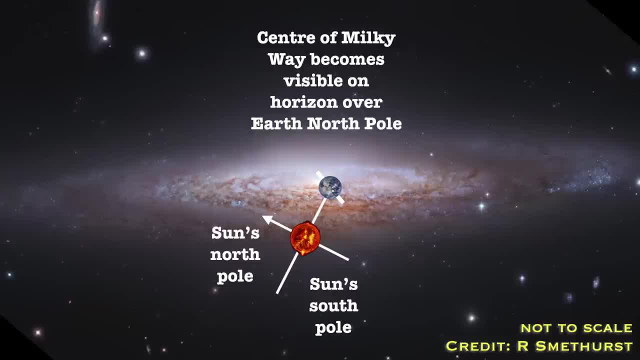 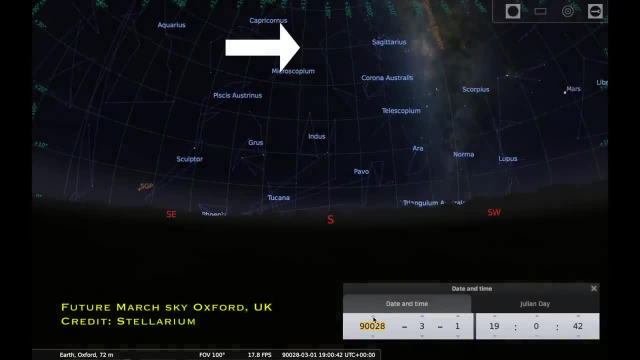 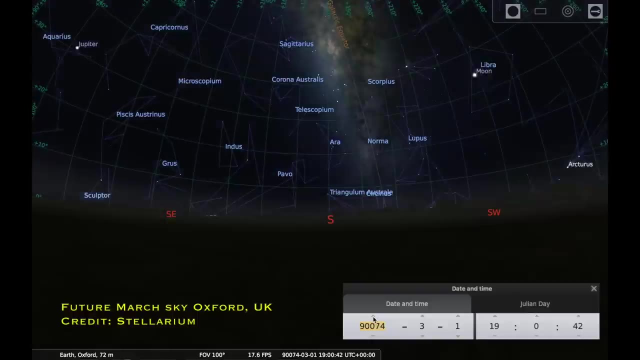 start to rise above the horizon at the north pole in 60 million years time. but all the time the sun keeps orbiting around the center of the milky way, sagittarius will rise higher and higher at latitudes similar to where i am in the uk, so that eventually, by the year 100 000, it will rise above. 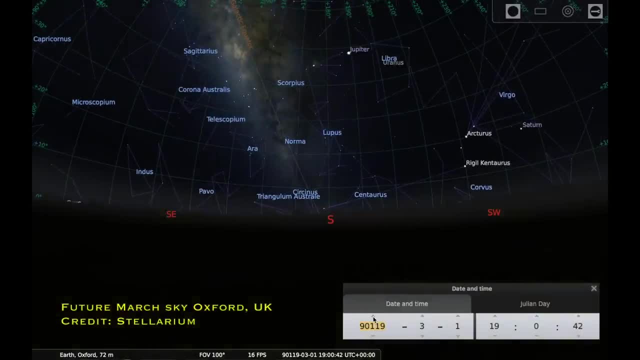 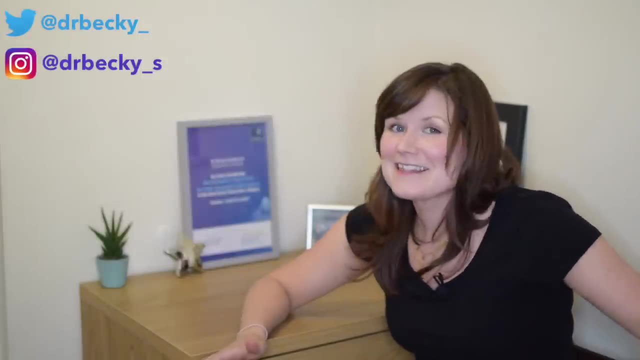 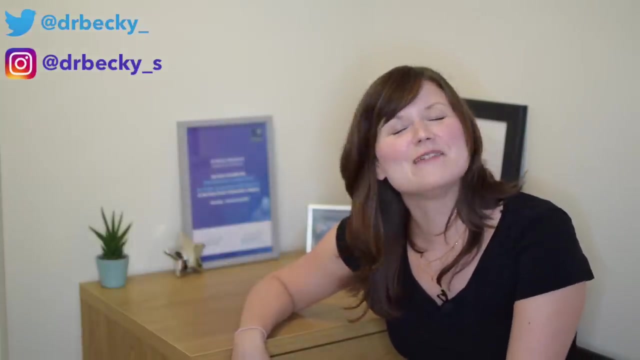 like 20 degrees in the sky, instead of just going up to the top of the moon and then going down to the springtime of each year so that i am actually able to appreciate it in all its glory. so all i need to do is live another 97 981 years and i will get my wish of being able to see the center of the milky. 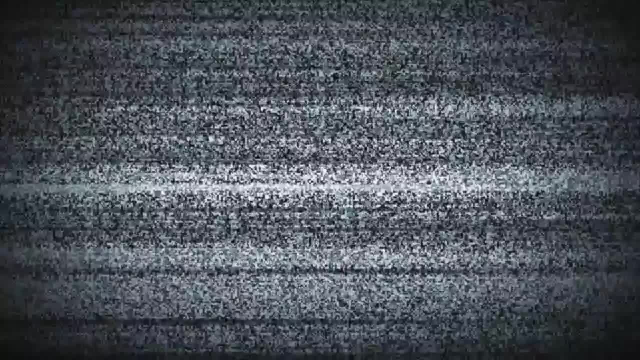 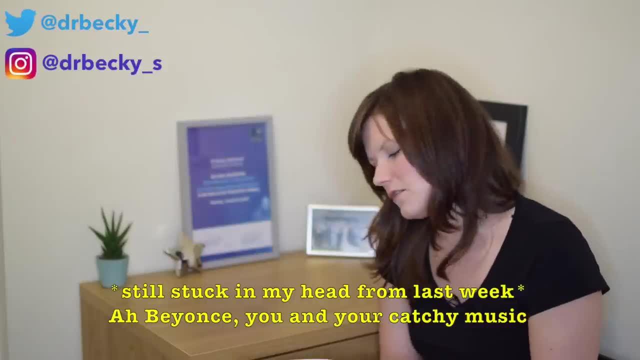 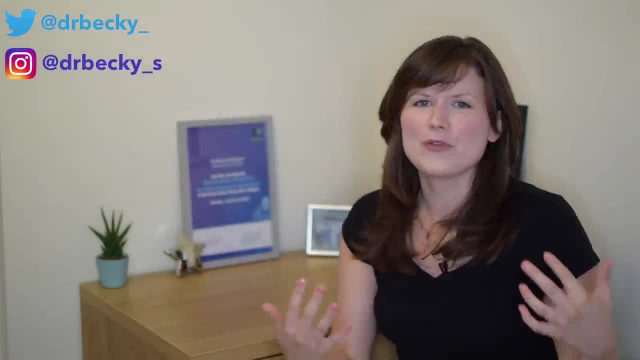 way from where i live in the northern hemisphere. brown skin girl, your skin, just like pearls, the best thing in the world. oh, excuse me, i need a holiday. you know, when you think about the earth growing the sun, the sun going around the center of the milky way, you often think about them as being 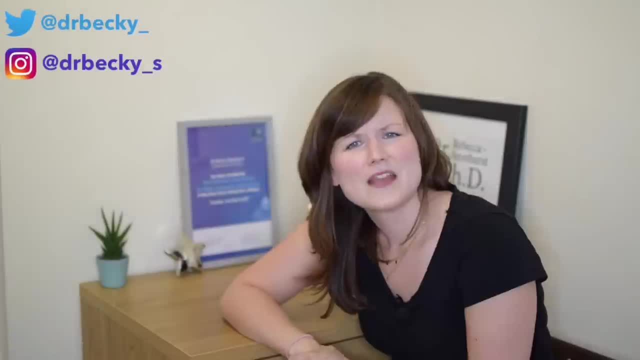 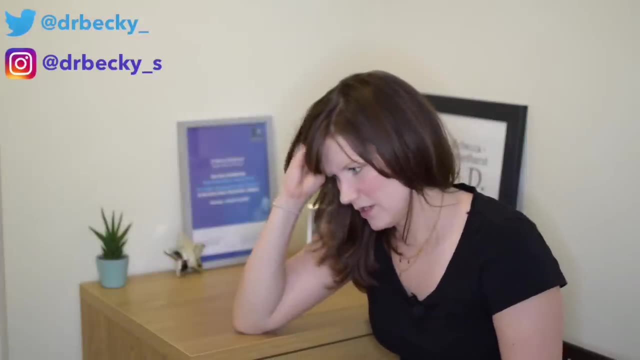 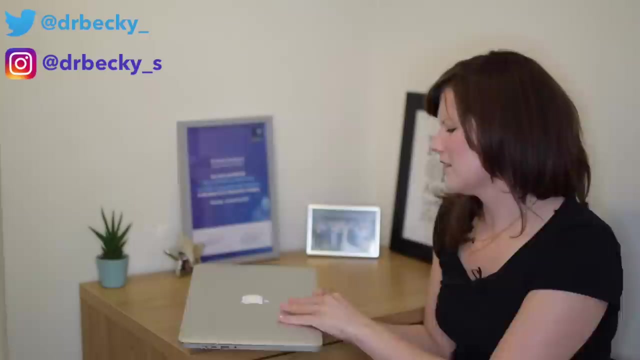 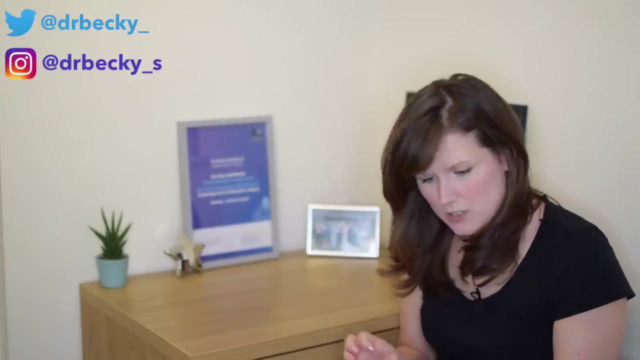 lined. so all i've got to do is live another 918, 2019 minus a hundred thousand hundred thousand minus 2019. nine, nine, nine, no, nine, eight, nine, seven. what should we do with the drunken sailor? what should we do with the drunken astronomer? what should we do with the drunken astronomer in the morning?